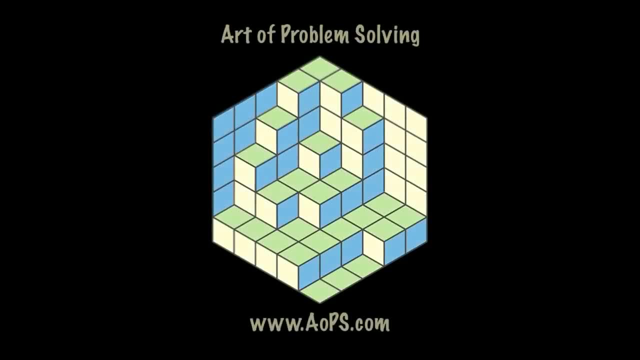 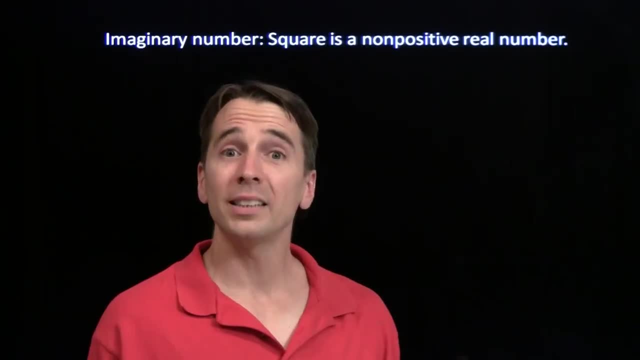 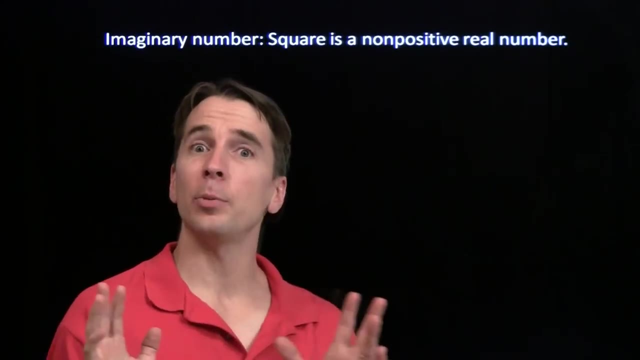 In our last couple lessons we came up with a whole new kind of number called an imaginary number. Now in this lesson we're going to keep on going, come up with something even more complicated. We're going to call that a complex number. But before we get to that, 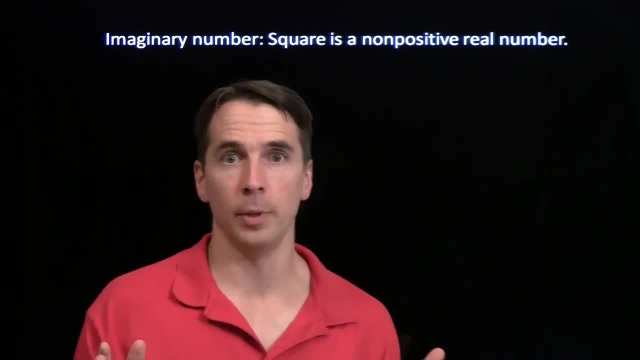 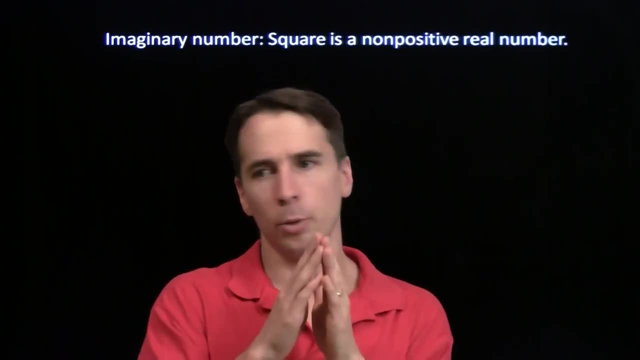 I want to talk a little bit more about imaginary numbers and how we came up with them. And before we even knew about imaginary numbers, all we knew about were the numbers on the number line. We called those the real numbers. There were negative numbers, there was zero. 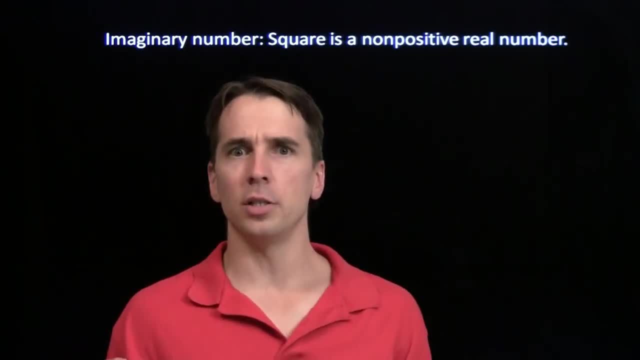 and there was a bunch of positive numbers. Then we started thinking about squaring these numbers. You square a negative number, you get a positive number. You square a positive number, you get a positive number. You square zero, you get zero. What do you square to? 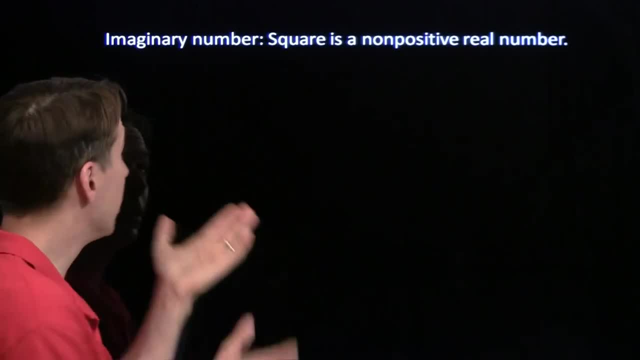 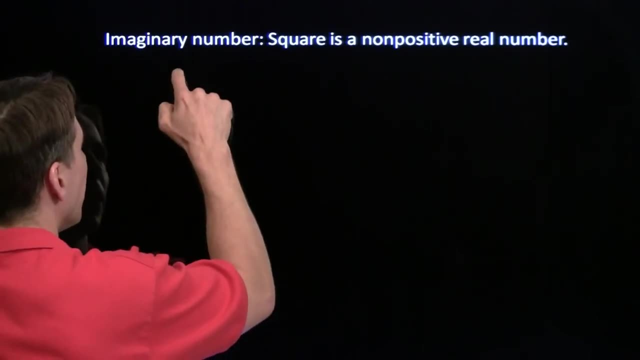 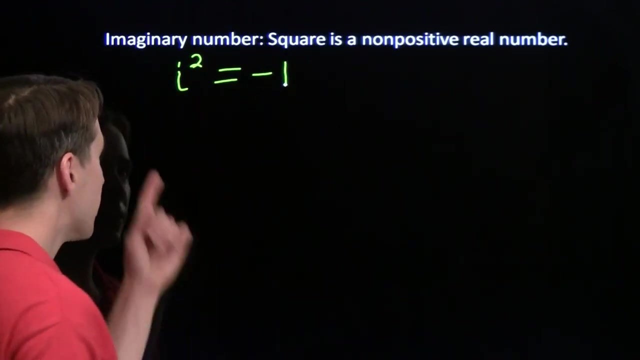 get negative numbers. That's where imaginary numbers come in. Imaginary numbers are the numbers whose squares are non-positive real numbers. And we started off by defining a whole new number we called i, and i is the number whose square is zero. i is negative, 1. And since the square of i is non-positive, it's negative. it tells us. 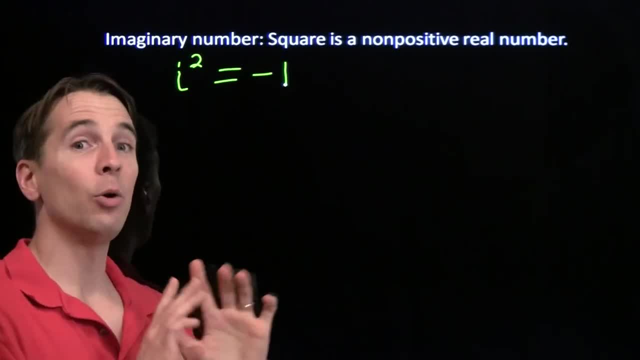 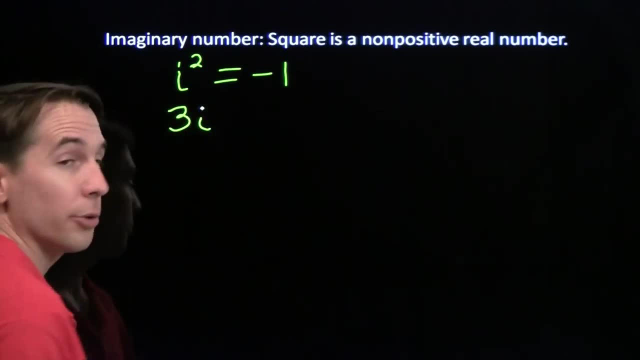 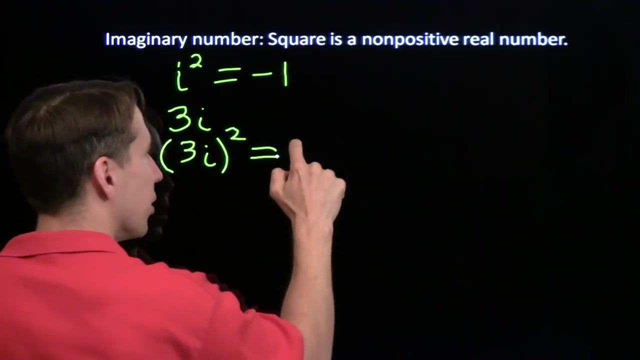 that i is imaginary. Now, i is not the only imaginary number that's out there. That's good for i, because i doesn't want to be lonely. Let's look at the number 3i- just 3 times i- And what happens when you square that? Now, if I square 3i, I get 3 squared times. 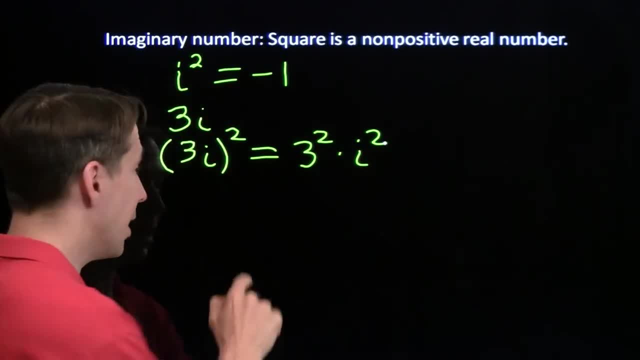 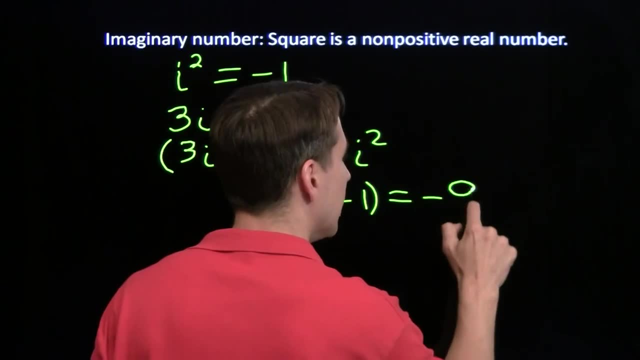 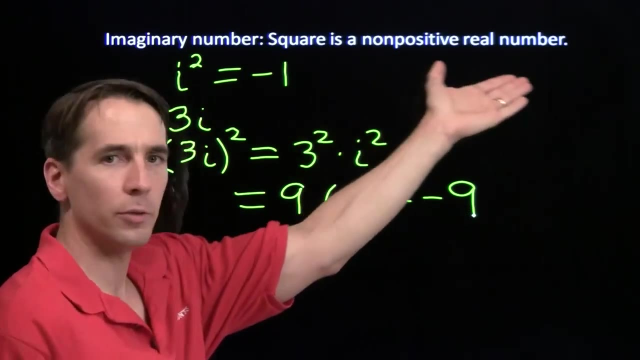 i squared And 3 squared is 9.. And of course we defined i squared to be negative 1.. 9 times negative 1 is negative 9.. So if I square 3i, I get a negative number, I get a non-positive real number And that 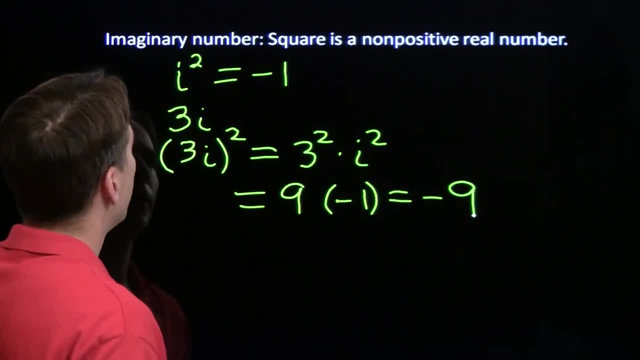 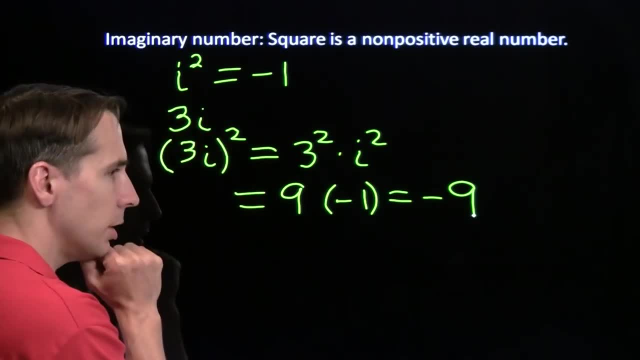 tells me that 3i is imaginary. All right, so let me see Now. where exactly do all these real numbers fit in? How do we compare them with the imaginary numbers? Well, the imaginary numbers. if you square an imaginary. 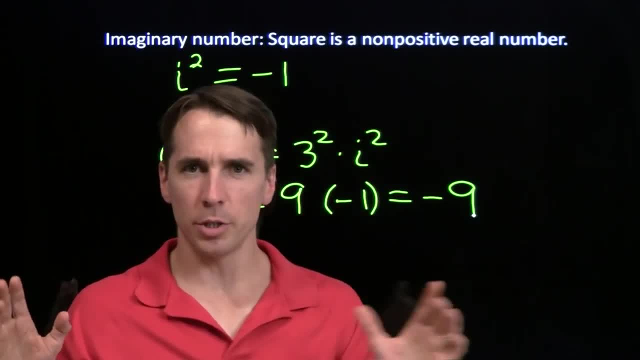 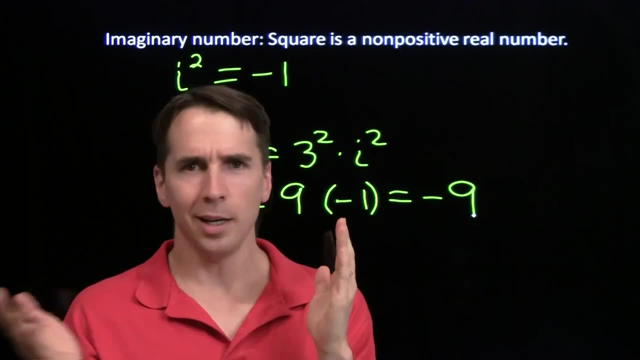 number, you get a non-positive real number. And what happens when you square real numbers? You square a negative, you get a positive, You square a positive, you get a positive. And if you square 0, you stay at 0. You can't. 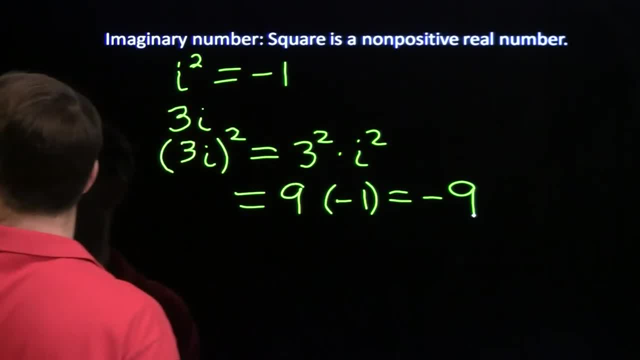 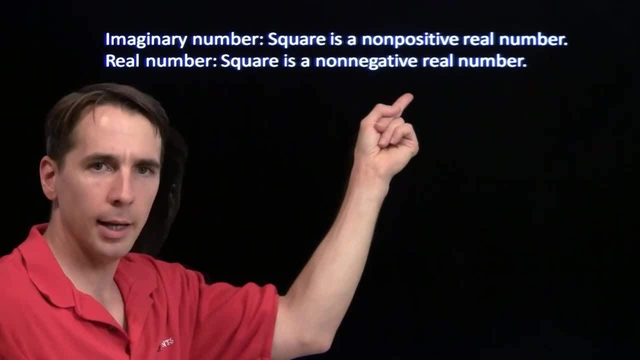 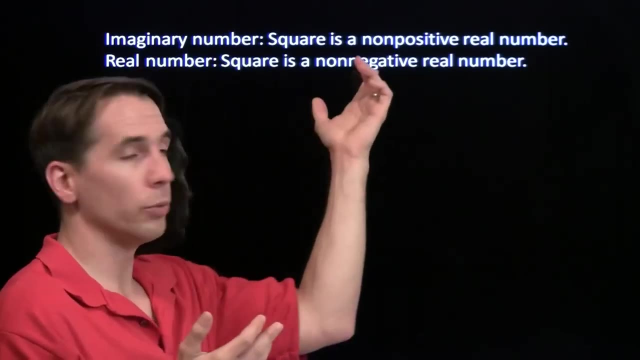 get negative numbers when you square reals. That's where the key distinction between these two is: If you square a real number, you get a non-negative real number. You can't get negative numbers If you square imaginary numbers. that's where you get non-positive. 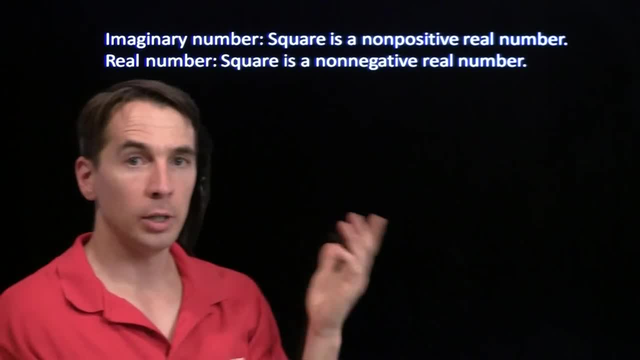 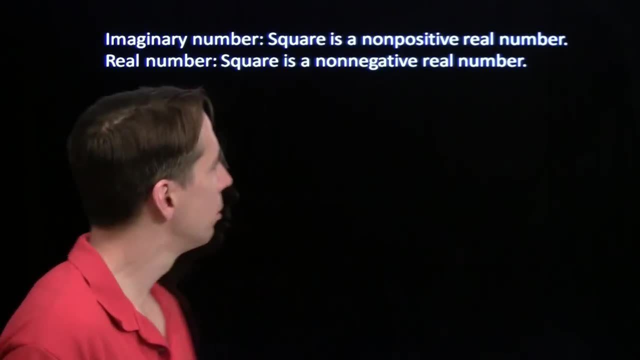 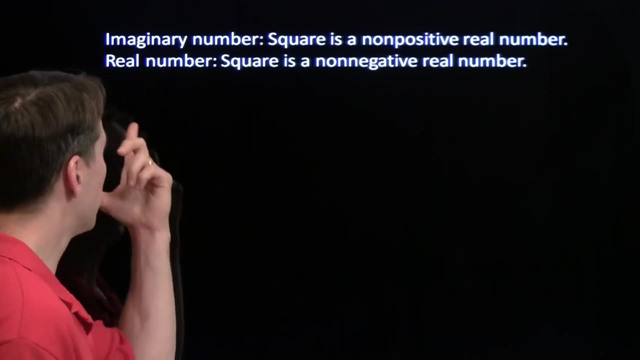 real numbers. You can't get a positive number when you square an imaginary number. You have. You have to get non-positive real numbers. Now wait a second. where does zero fit in? Zero is not positive, zero is not negative. so is it real or is it imaginary? 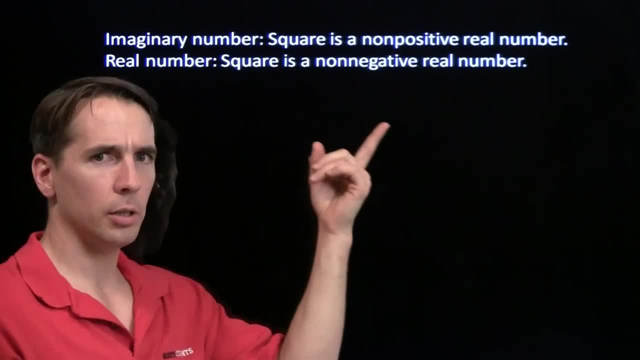 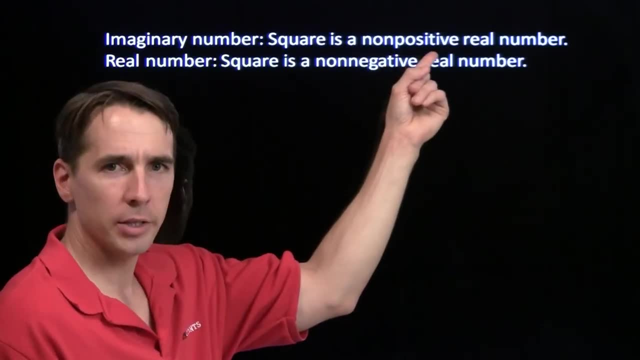 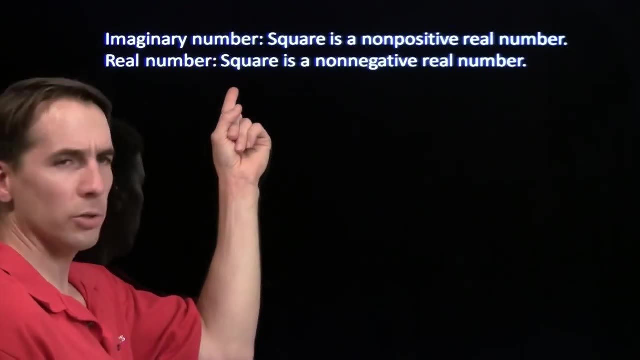 Let's think this through: Zero squared is zero, and zero is not positive, So the square of zero is not positive, so zero is imaginary. Wait a second: zero squared is still zero and zero is not negative. so the square of 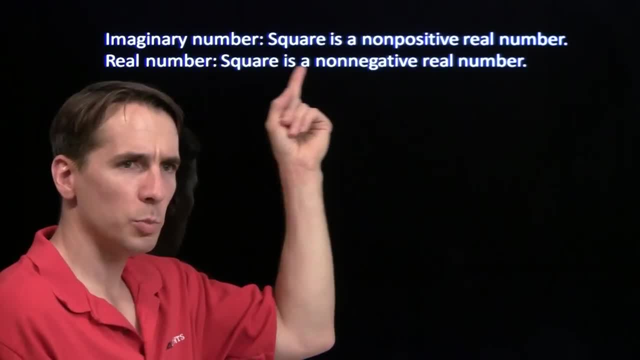 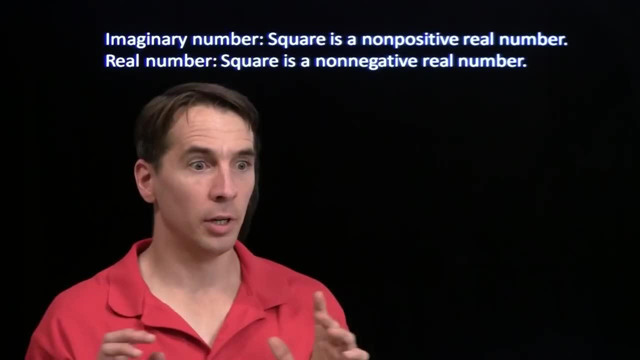 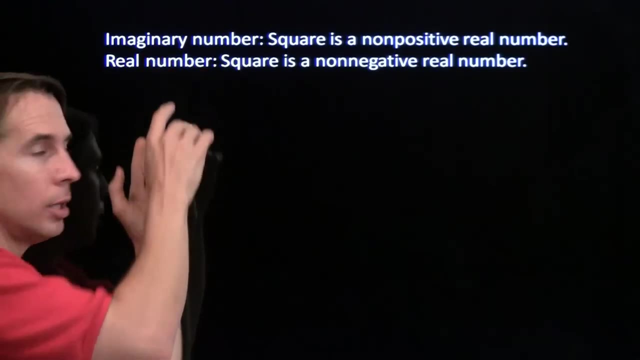 zero is not negative either, which means zero is real. Aha, Just like zero is not positive and it's not negative, zero is both real and imaginary. So there's one number out there that's both real and imaginary, and that's zero. 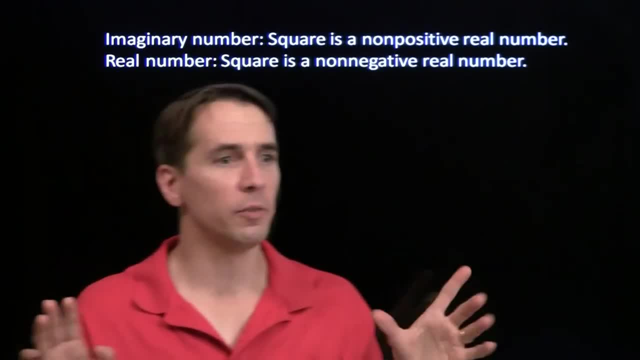 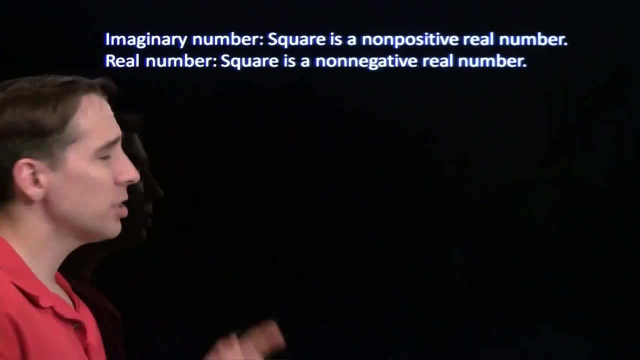 All right, we got this down now. Real numbers: those are all the numbers we've always thought about before we ever even knew about imaginary numbers. Numbers on the number line- there's no i anywhere. The imaginary numbers: those are the numbers that we get when we take one of these real. 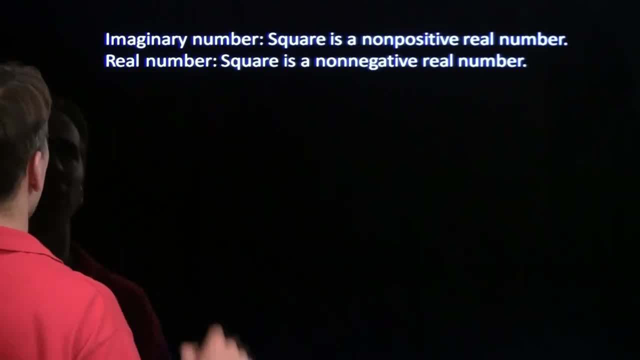 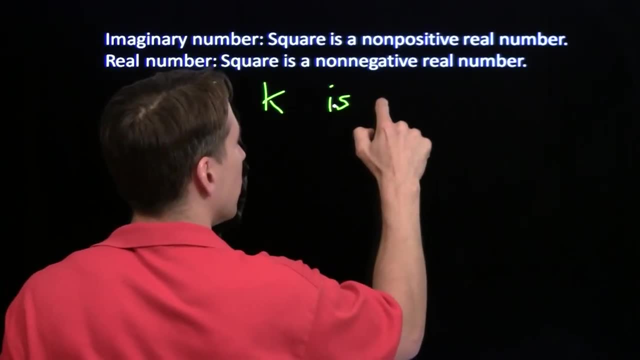 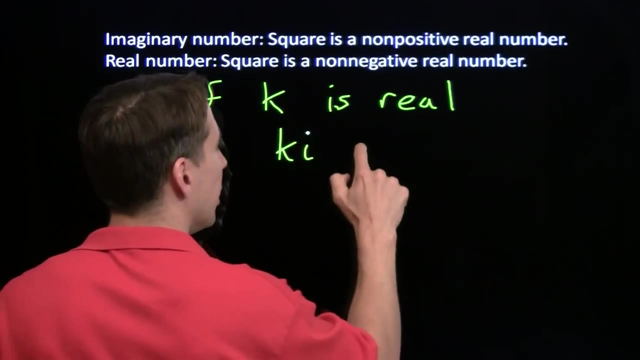 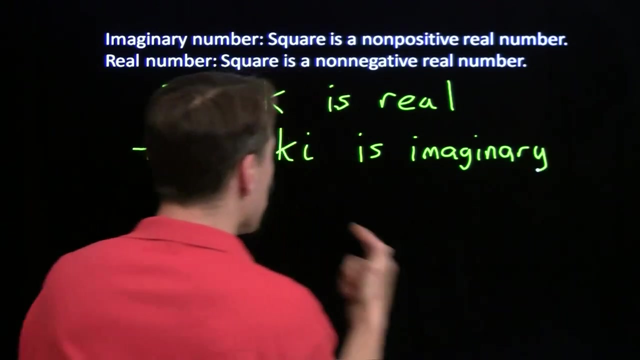 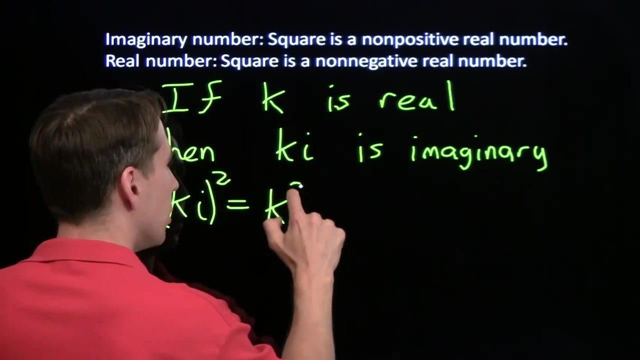 numbers and we multiply it by i, We can check this out just like this: Say that k is some real number, Then k times i is imaginary. and we can see why just by squaring this. If we square k times i, we get k squared times i squared, and of course i squared is negative. 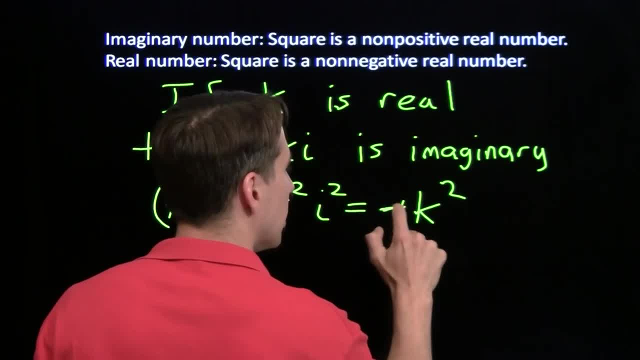 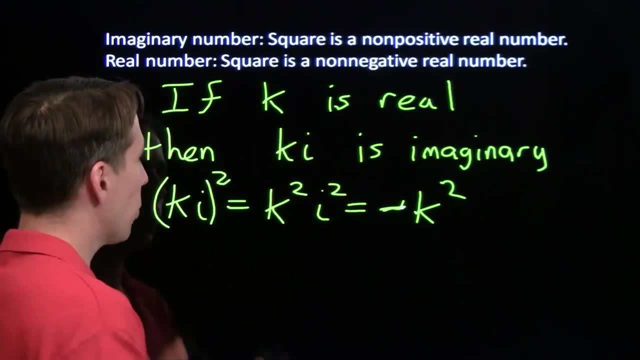 1. So we get negative. 1. So we get negative k squared and k is a real number. so minus k squared, that's non-positive. So when we square k i, we get a non-positive real number that tells us that k i is imaginary. 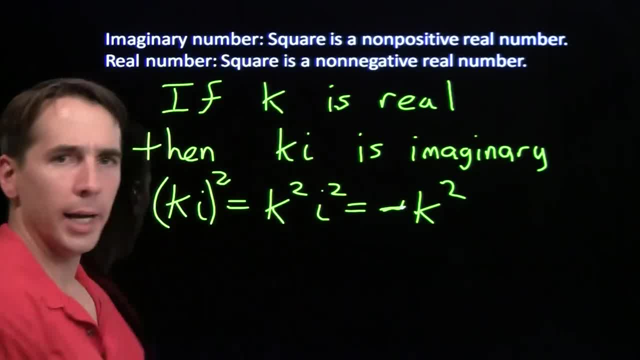 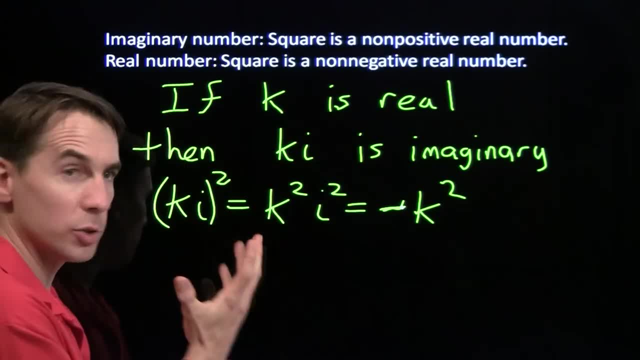 All right. so now we know how to tell if we've got something that's real. there's no i anywhere. And if we take a real times i, that gives us an imaginary number And zero is both. If I put zero in there, it doesn't have an i- and zero times i. that goes back to zero. 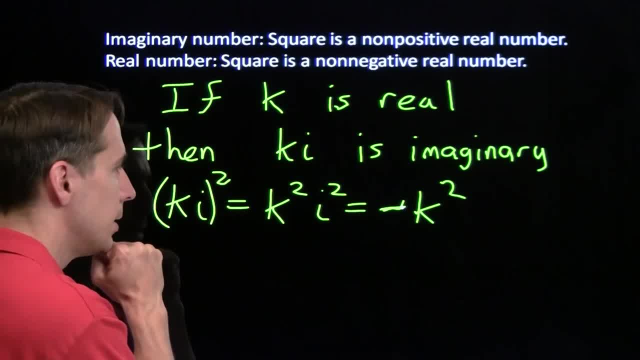 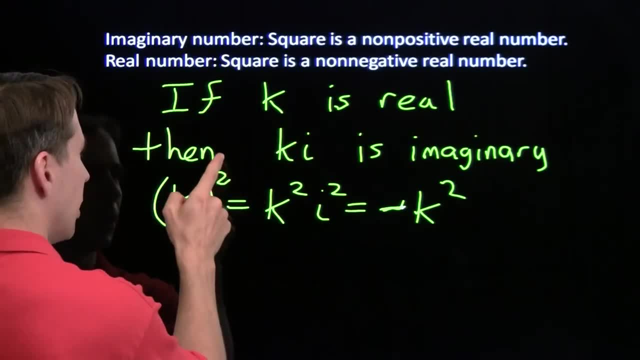 but that's still something times i. Zero is real and imaginary. It's still a little weird, but hmm, we'll come back to thinking about that in a minute, Because first I want to add some of these numbers up. We know how to add real numbers. 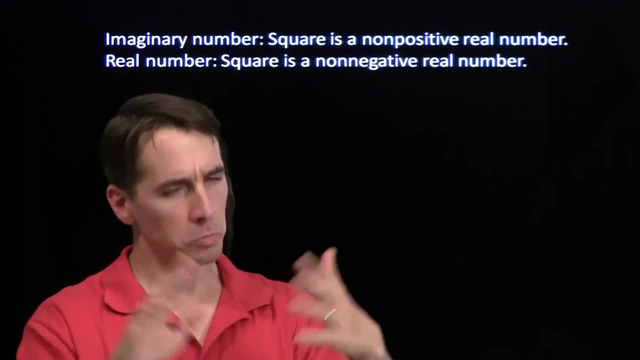 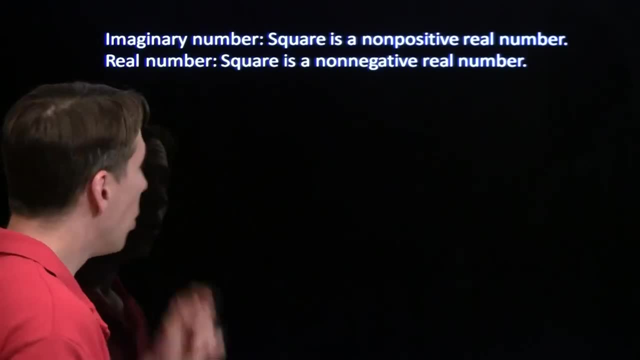 Two plus three, That's five. That's easy. Add two real numbers, you get another real number, because an i isn't going to magically pop up out of somewhere. So we add two real numbers, we get a real number. 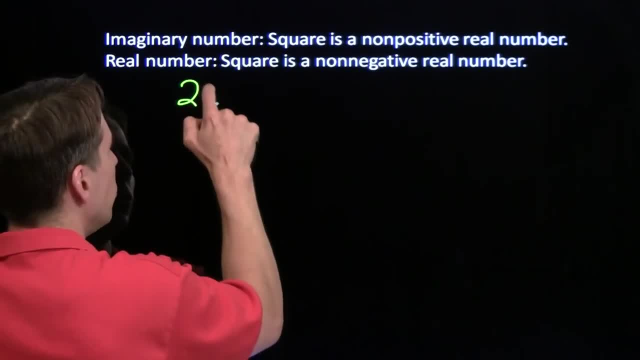 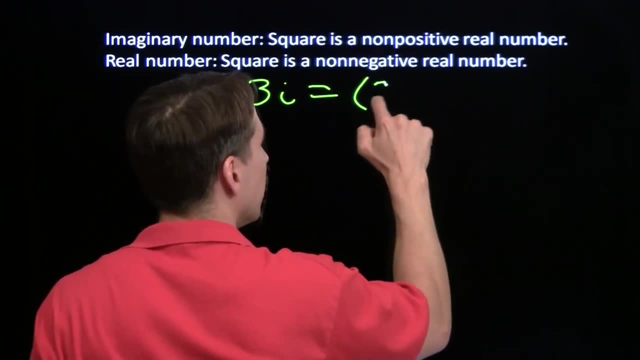 What about adding two imaginary numbers? So we take two i plus three i. Now we use a little distributive property here. We factor out the i and we get two plus three times i and the sum two plus three, of course. 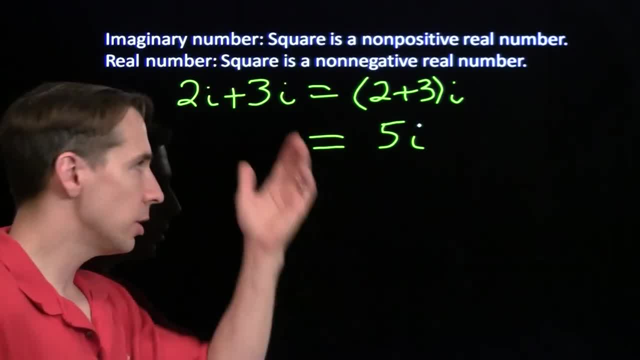 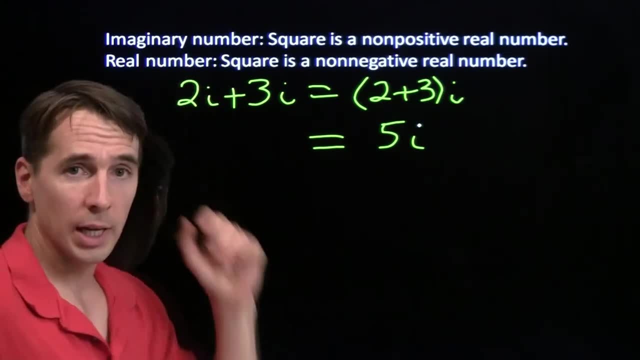 is five, We have five, i So sure enough. you add two imaginary numbers, you get another imaginary number. Not surprising at all. We add two real numbers, we get a real number. We add two imaginary numbers, we get an imaginary number. 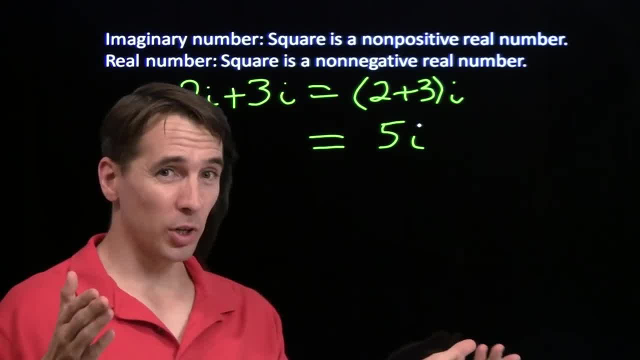 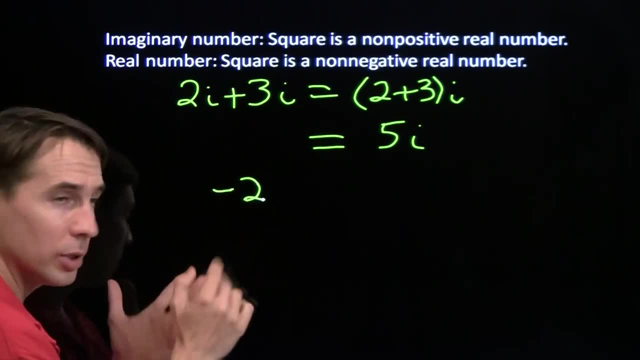 You know what we're going to look at next. What happens if we add a real number, Add an imaginary number? What happens if we take a number like negative two- that's a nice real number- and we add it to three, i, which is an imaginary number? 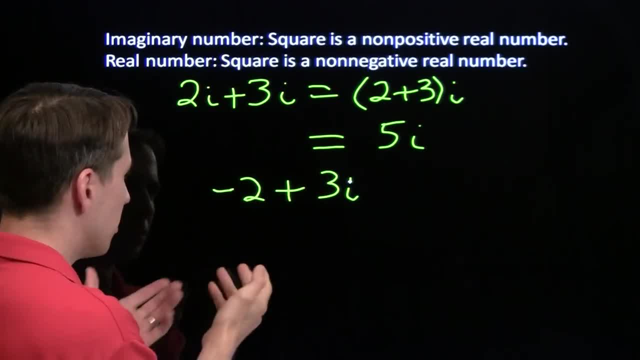 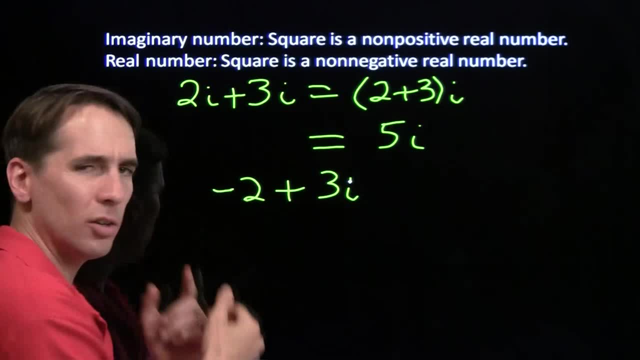 What's that? Well, it's not a real number because it's got that i sitting in there. But it's not just some real number- times i- because it's got this thing over here, so it doesn't look like an imaginary number either. 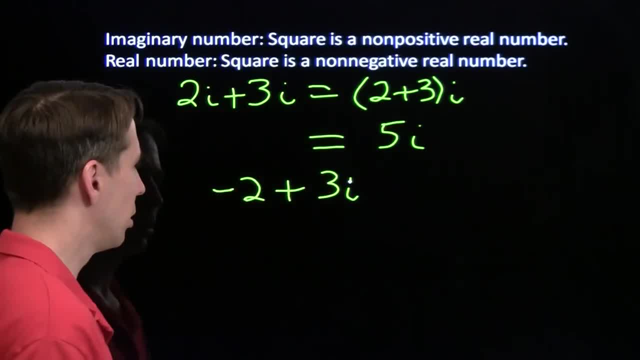 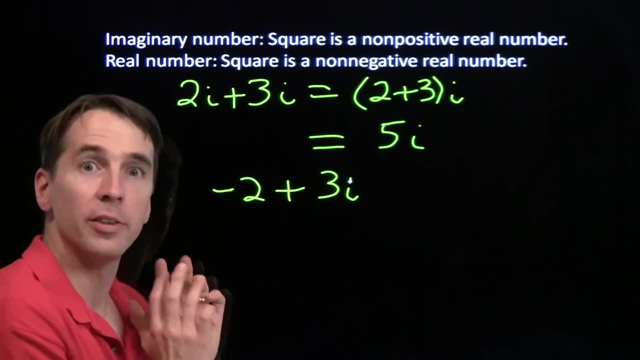 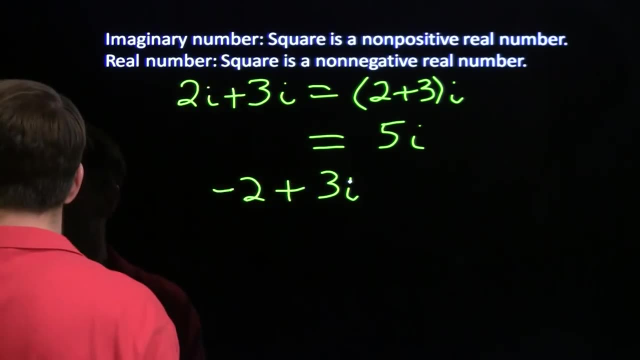 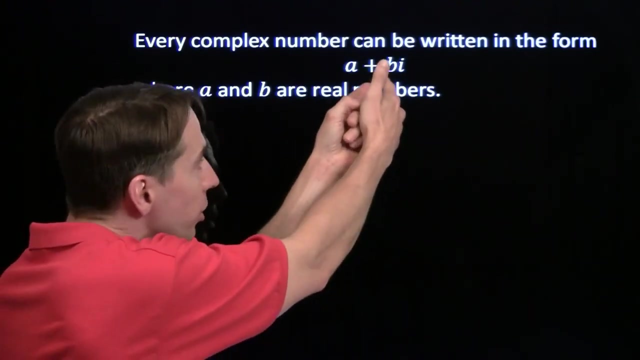 I can't simplify it like I did up here. Well, this is complicated. This is so complicated that we invent a whole new number type just for this. We call it a complex number. This is what we call a complex number, And a complex number is a real number, a plus some real number times, i plus bi here. 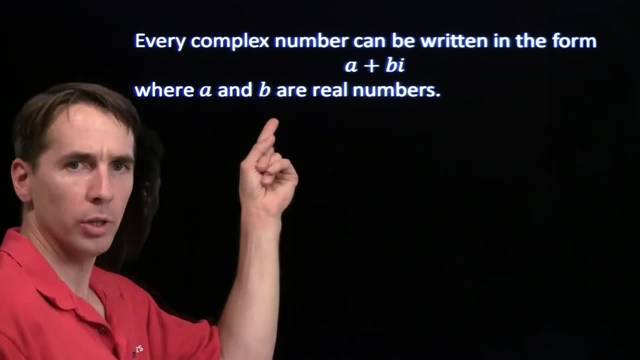 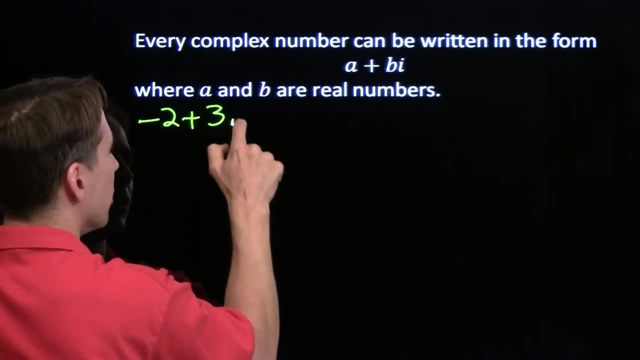 Any complex number is in this form, a plus bi, where a and b are real numbers. Now let's take a question. Let's take a closer look at that negative two plus three i. with this definition, Negative two plus three i, that's a complex number. 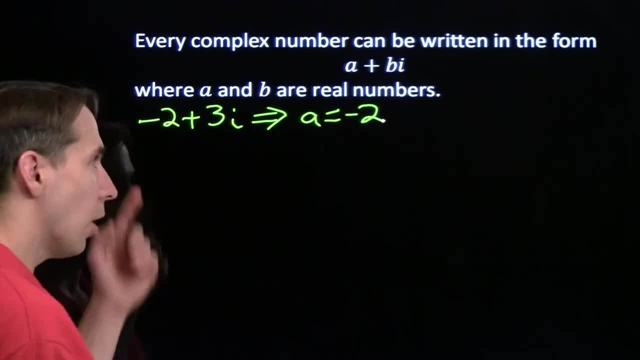 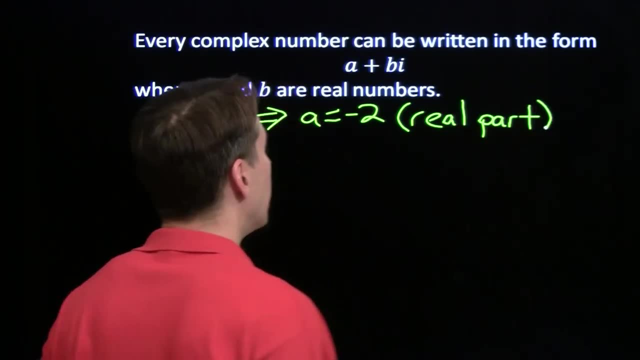 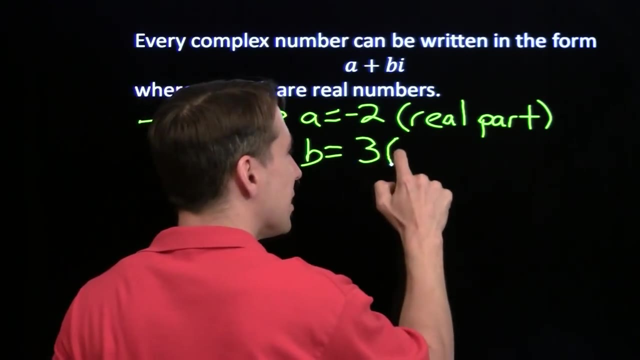 And here a is negative two, and we call that the real part, And b, while it's the number that we multiply by i, b, is three, And we call that the real part, And b, while it's the number that we multiply by i. b is three. 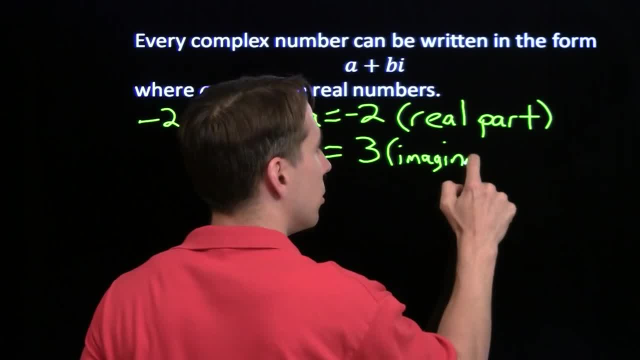 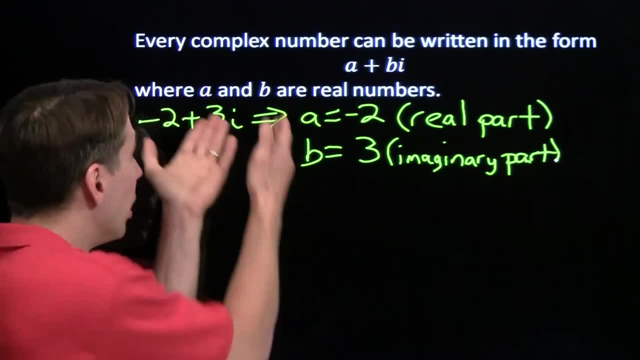 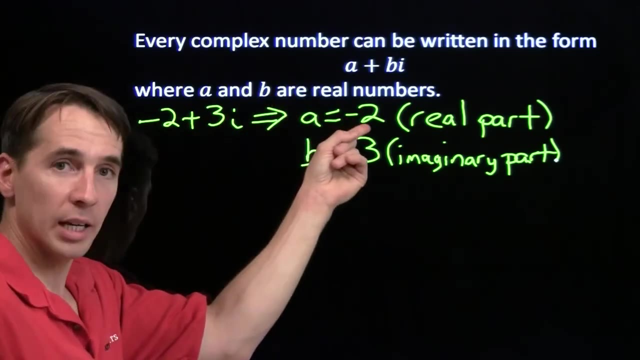 And b is the imaginary part. Now one subtle point here: the imaginary part is a real number. That's the real number that we're multiplying by i in our complex number. So negative two plus three i: the real part is the negative two. 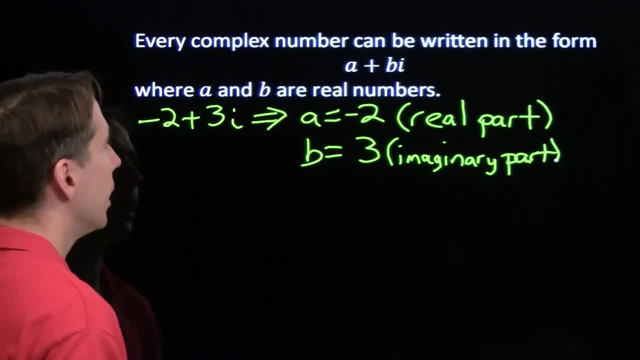 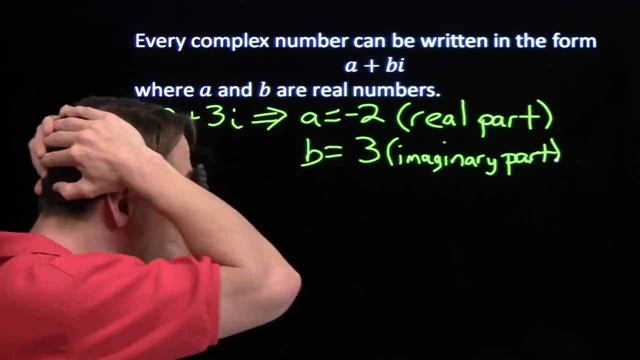 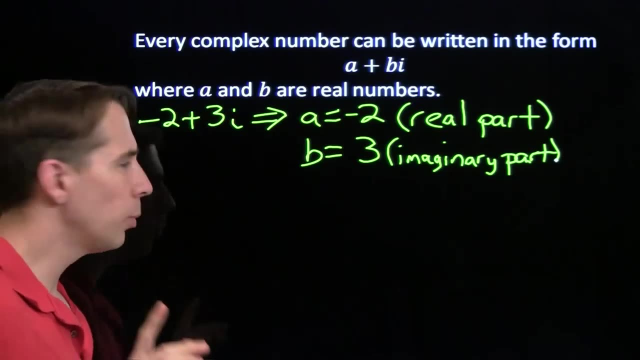 And the imaginary part is the three, not the three i. So now I've got complex numbers and imaginary numbers. We've got real numbers. How do these things all fit together? Okay, Hey, wait a second, let's take a look at one of these. just a real number, 5.. 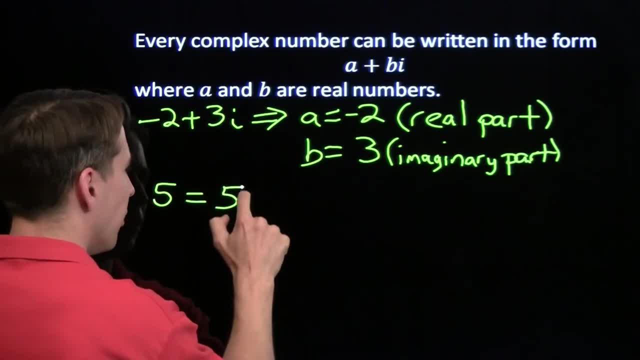 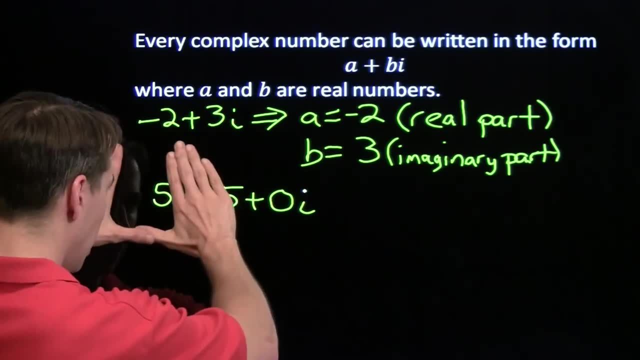 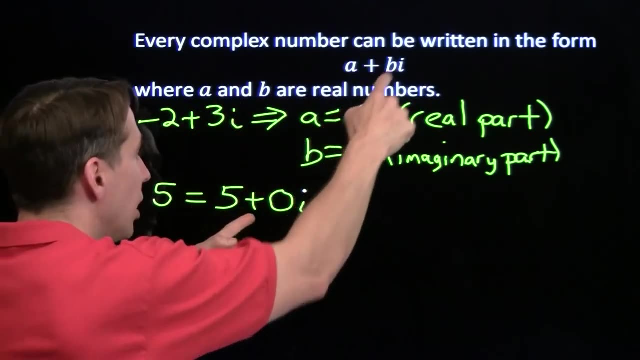 I can write 5 as 5 plus 0i, So 5, this is a real number. This over here, 5 plus 0i, is a complex number because it's just in this form: a is 5, b is 0.. 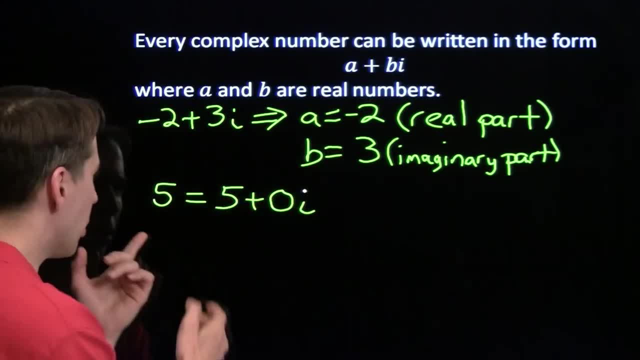 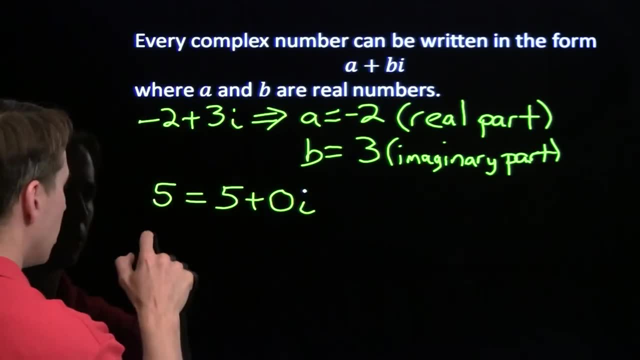 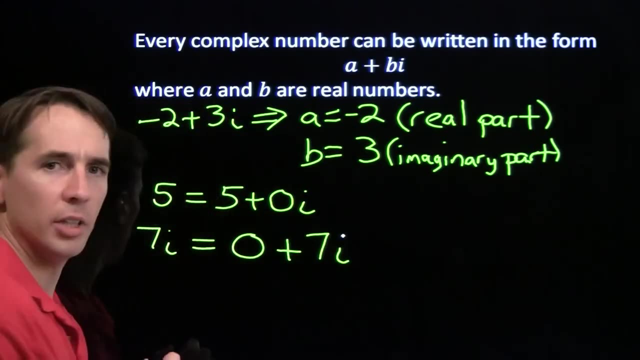 That's a complex number. These two are the same because 0 times i is just 0. So real numbers are complex numbers. What about imaginary numbers? We take 7i and that's just 0 plus 7i. 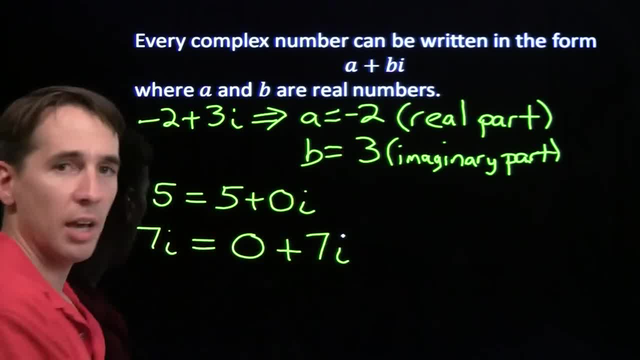 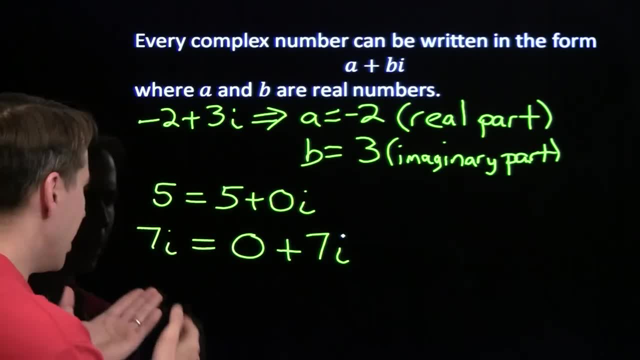 Well, that's a complex number. a is 0,, b is 7, and 0 plus 7i. well, that's the same thing as 7i, which we know. 7i is an imaginary number. You square that, you get negative 49.. 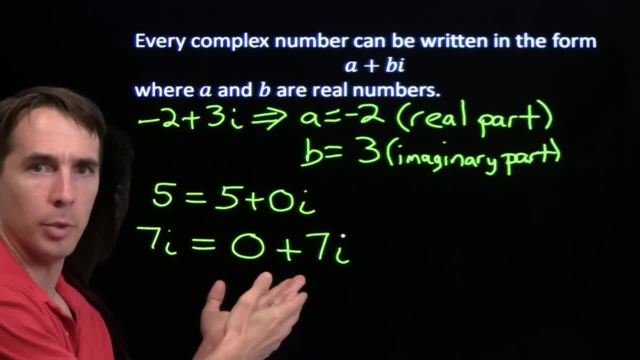 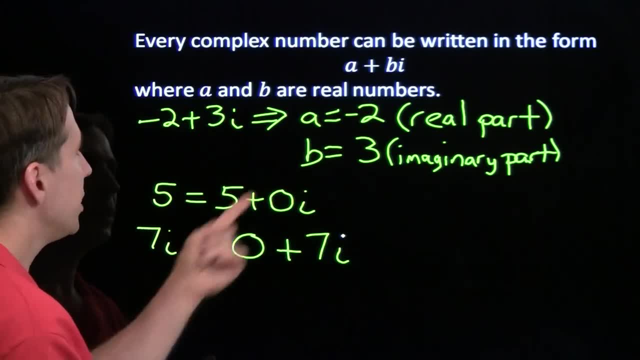 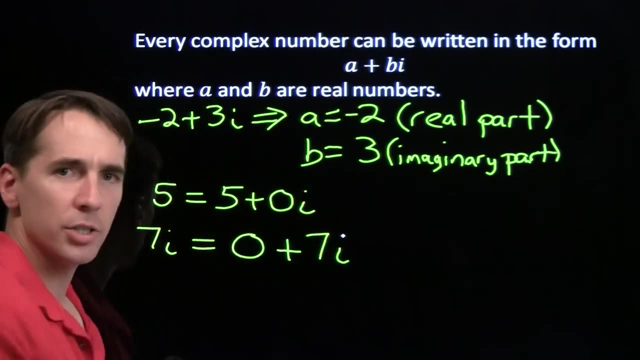 So imaginary numbers are also complex numbers. So real numbers and imaginary numbers are just special cases of complex numbers. Anytime b is 0, we end up with a real number. Anytime a is 0, we end up with an imaginary number. 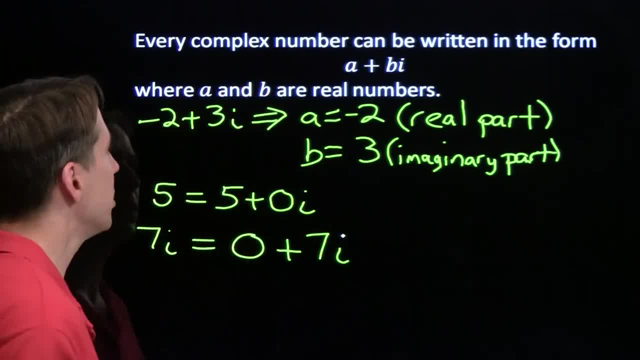 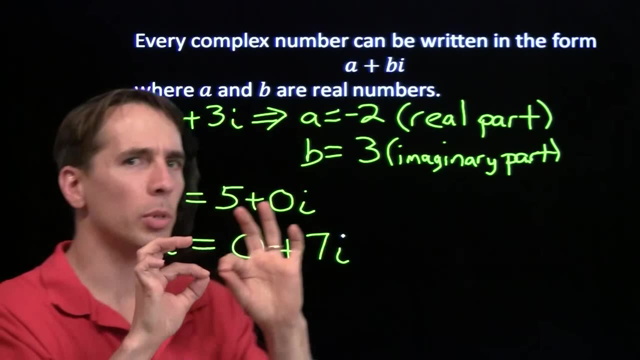 So real numbers and imaginary numbers are just special cases of complex numbers. Still, there's this thing right here which is definitely not real and it doesn't look like it's imaginary either. How do we think about these new numbers? Well, we can't put them on a number line anymore, right? 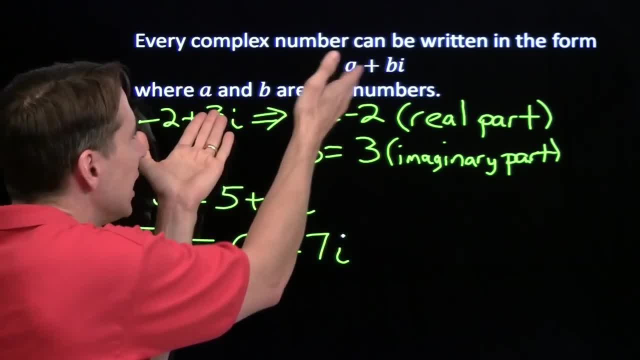 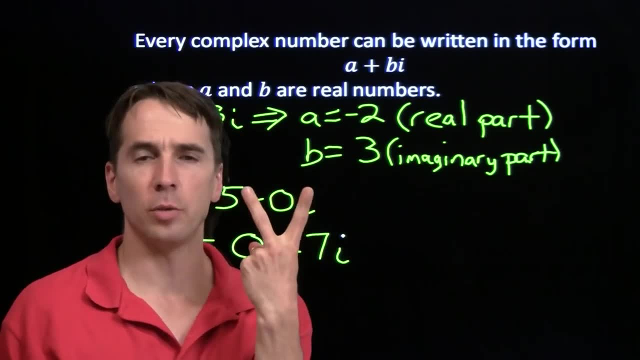 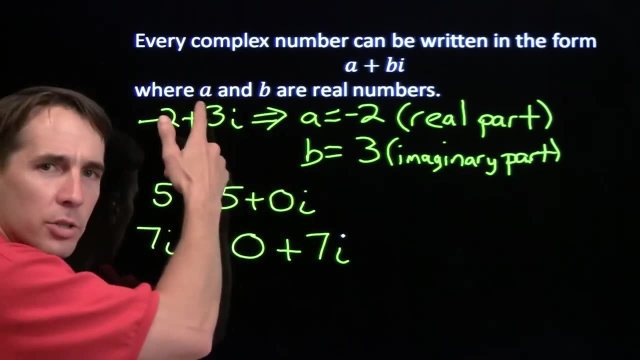 With a number line. a number line just have one number. Here we're defining each complex number in terms of two real numbers. Now where else have we seen things that were defined in terms of two real numbers? The Cartesian plane coordinates. We can draw pictures of complex numbers on a plane. 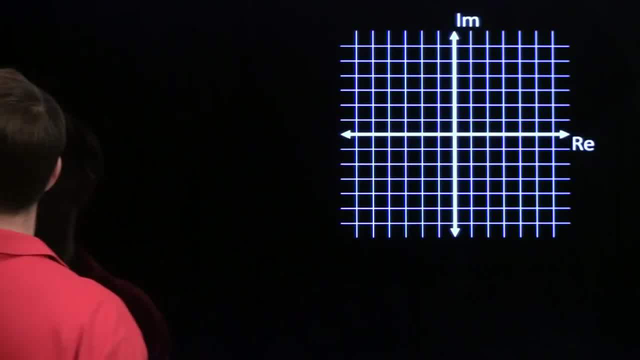 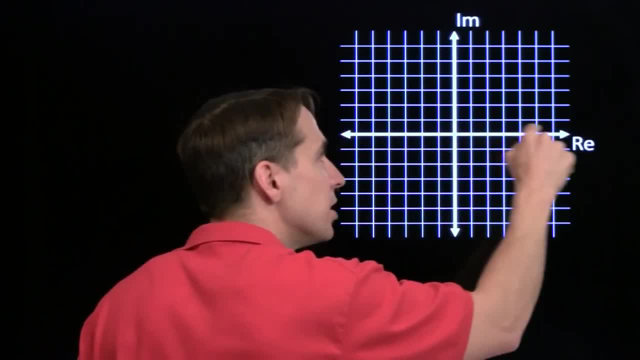 Just like we used to do real numbers on a number line with complex numbers, we can plot them on a whole plane. We have a real axis. we call this the real axis, and this is where all the real numbers are, And it's the same thing as the good old number lines. 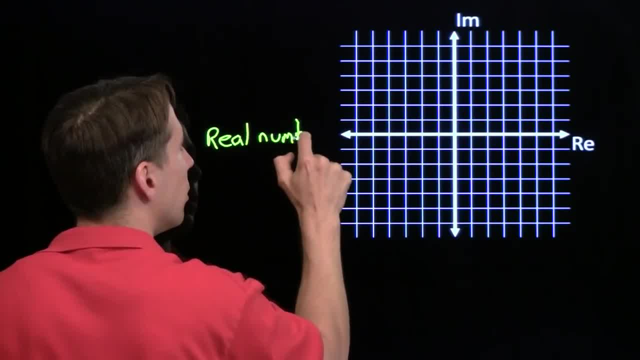 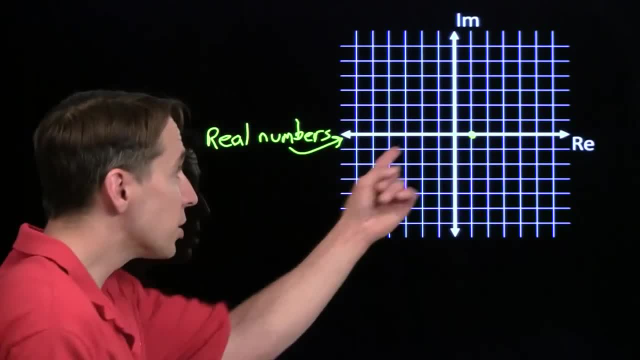 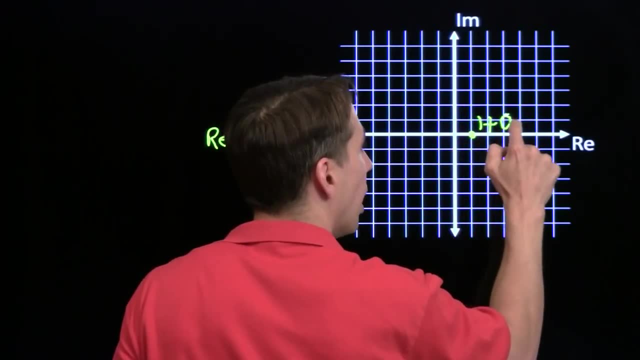 So the real numbers are right here. That's the real axis. So this number right here, that's 1.. The real part is 1.. The imaginary part is 0. We're not going up or down at all. This is 1 plus 0i, which you know as 1.. 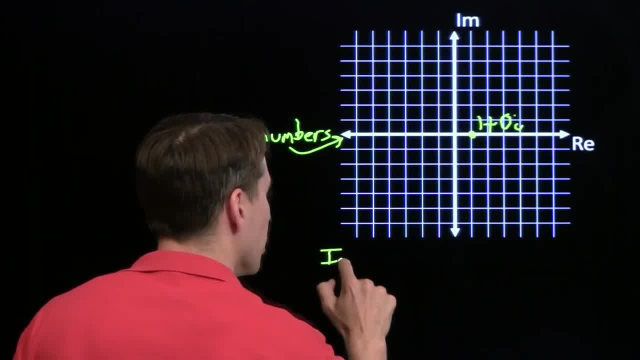 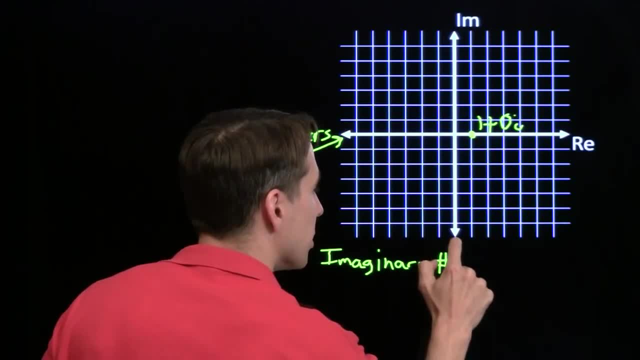 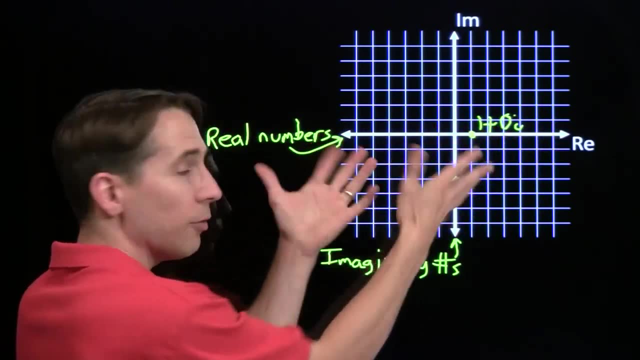 And then this axis: here these are the imaginary numbers Plotting the imaginary part vertically. it's this axis, So this point right here, for example, that in the real way going right or left, we don't go right or left at all, so that's 0.. 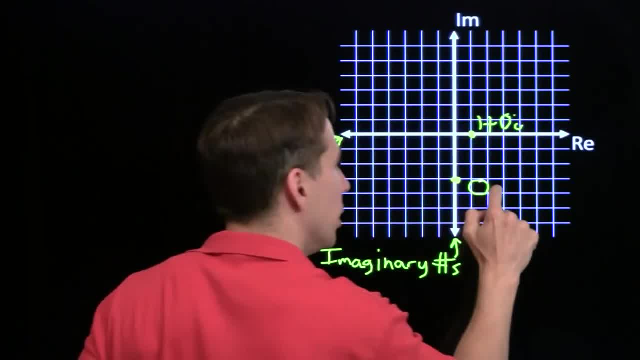 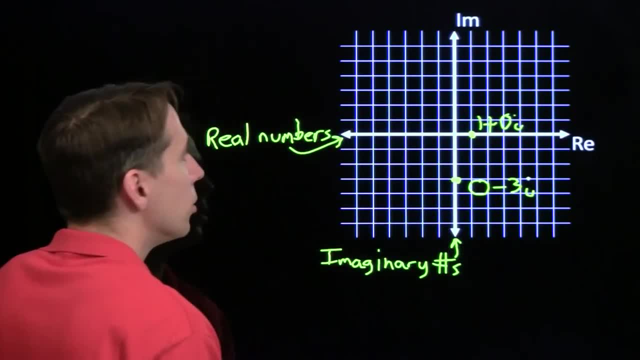 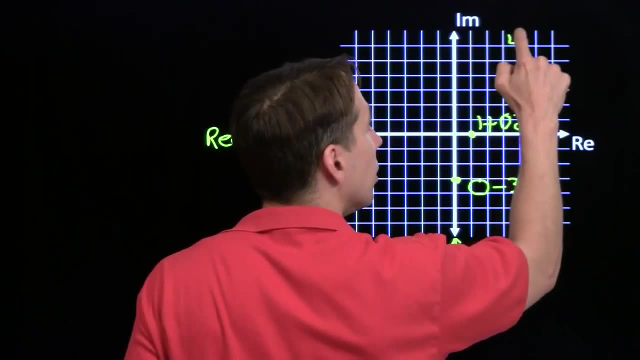 The real part is 0. And the imaginary part. Well, we go down 3 minus 3i, So that is the imaginary number minus 3i. So what about this number? up here We're going over 4, 1,, 2,, 3,, 4, and up 5, 1, 2,, 3,, 4,, 5, plus 5i.